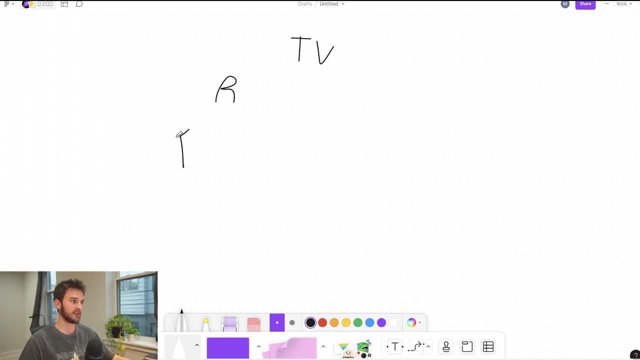 commonly like digital advertising platforms like YouTube ads or Facebook ads or meta ads or even Google ads, you know, even like different affiliate websites or things like that: apps. even So, any type of space where you can buy media And the goal is to effectively channel these people from. 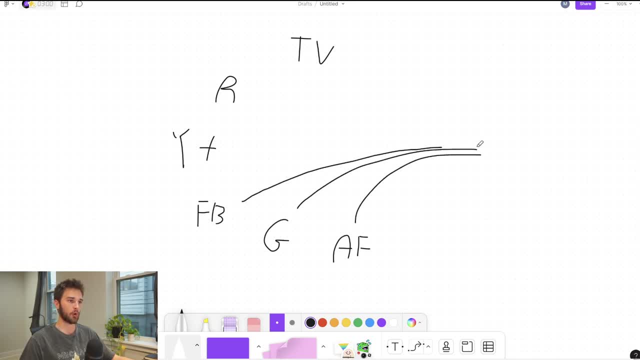 all these different places into a product or a funnel or into, ultimately, a business. And if you do this successfully, that's when you'll be able to grow the business. And this is literally what you'll look like as well, when you do this successfully, And that's when you'll be able to grow the business. 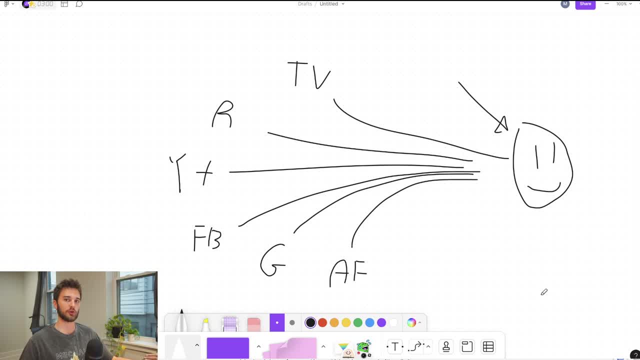 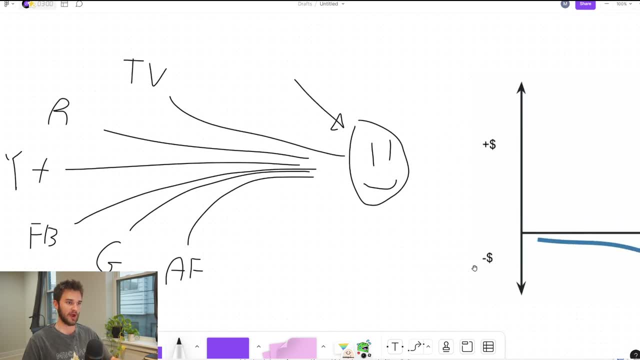 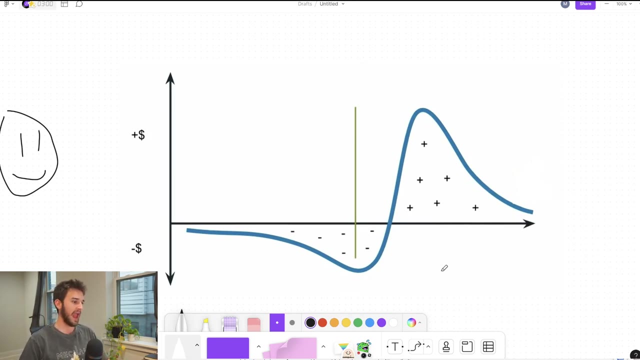 And, in other words, a media buyer is somebody who's a catalyst, It's somebody who can create asymmetrical returns, And this is something that I've learned and observed over time from Sam Ovens, the Beckers, the Harmosys, all those fun guys, And, in other words, 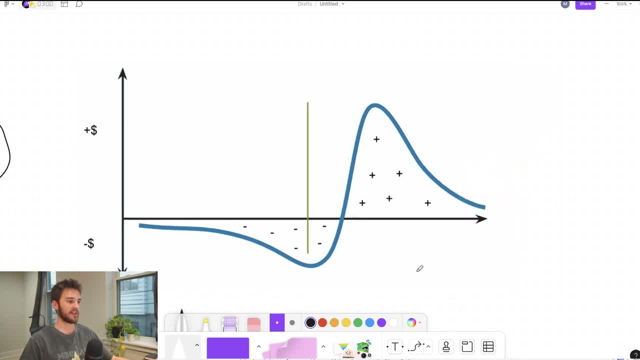 it comes down to this graph right here, And what this means is that there's an asymmetrical risk reward, where the risk is minimal and the chance for reward is very high, with uncapped or no limits And the best investors and media buyers and marketers in the world. 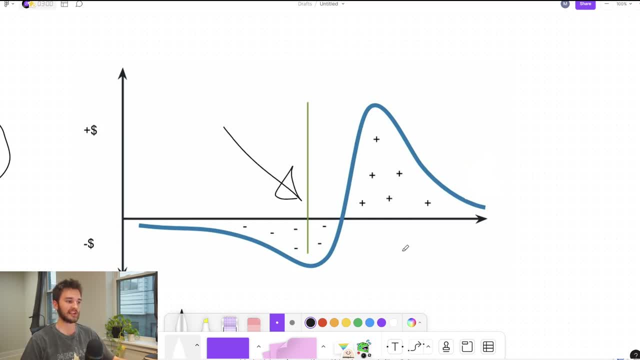 are very good at this, at creating this. This is also why it's so hard to find the best media buyers in the world and why the best media buyers are usually running their own show or running their own business or something. And that kind of brings me to my second point about defining. 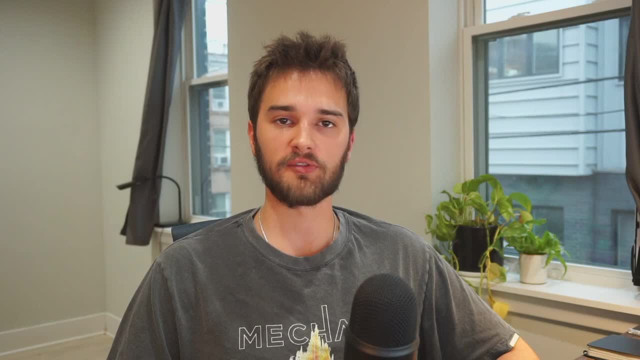 a media buyer and really the role of one. You know, if you're trying to provide mega value for a business or for your own business, you're not going to be able to find the best media buyers in the world. You're not going to be able to find the best media buyers in the world. You can't have. 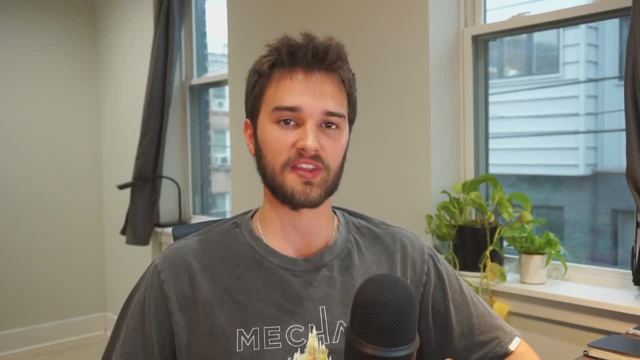 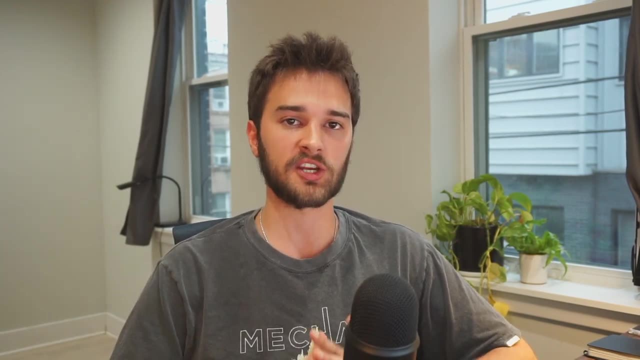 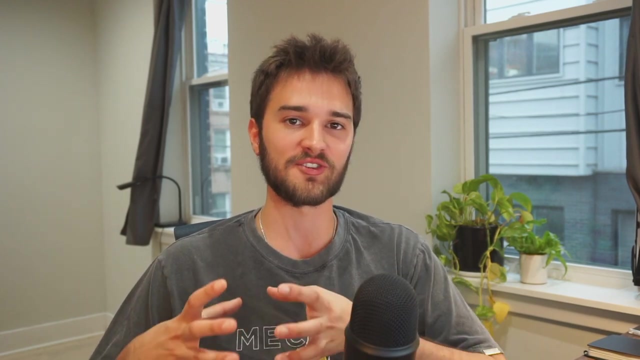 a button pusher, You need somebody who is much, much more than that. And when you look at the most capable media buyers out there, who you know really are killers, they're usually extremely full stack or very T-shaped, So they're not only going to be killers and savages inside of the ad. 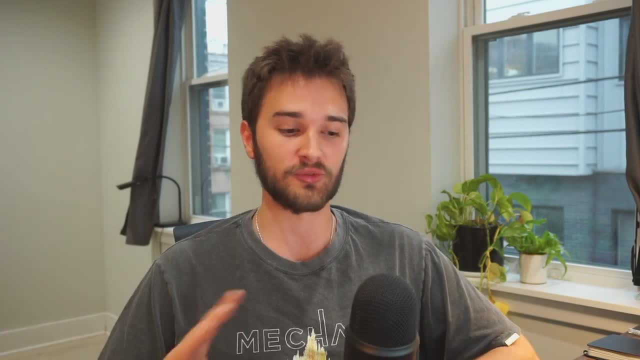 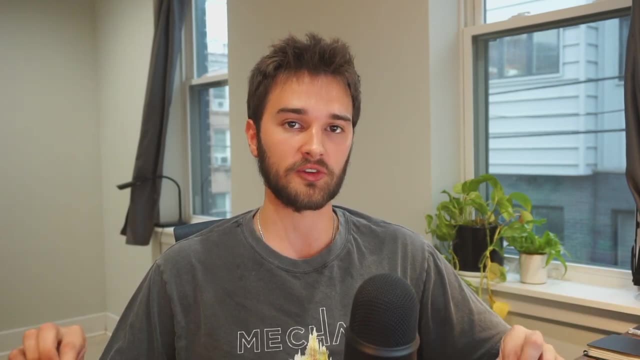 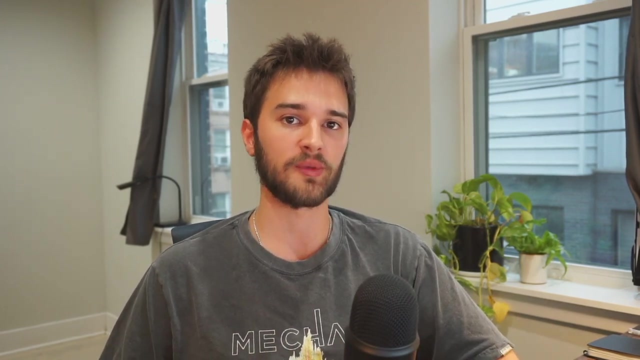 manager. you know whether it's Facebook ads or Google ads, YouTube, so on, But they're usually also going to be able to see all of those other interconnected constituent parts that still relate to advertising, whether it's email marketing or funnel building, conversion rate optimization, psychology, copywriting, but then even things 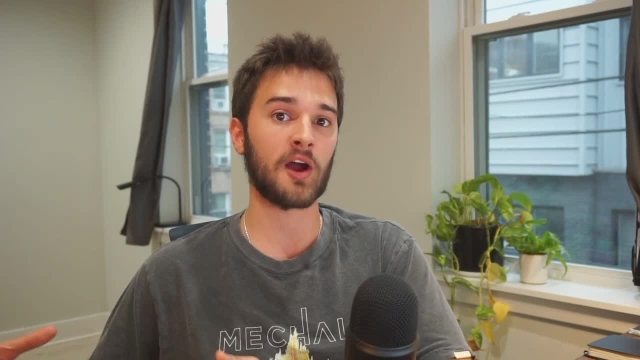 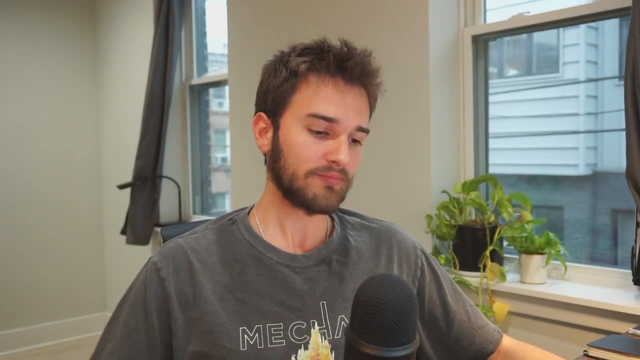 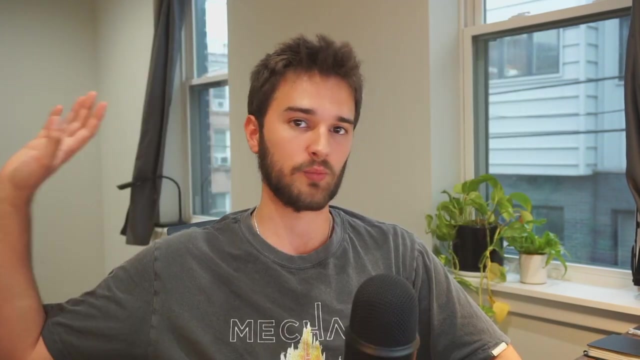 like finance things that maybe on first glance you might not really think that they go hand in hand together, but they do. And a really good example of this: you know I've been working with Alex Becker at Hyrus for years- and one of his webinar funnels like again. 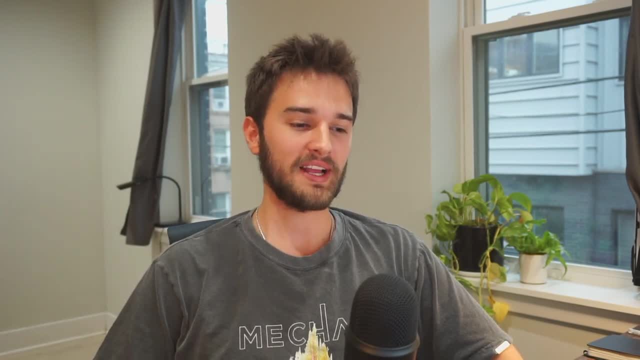 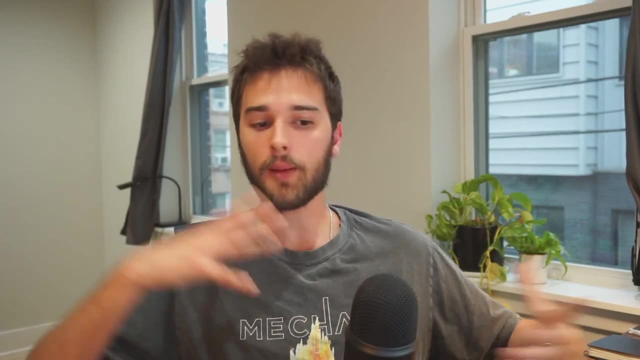 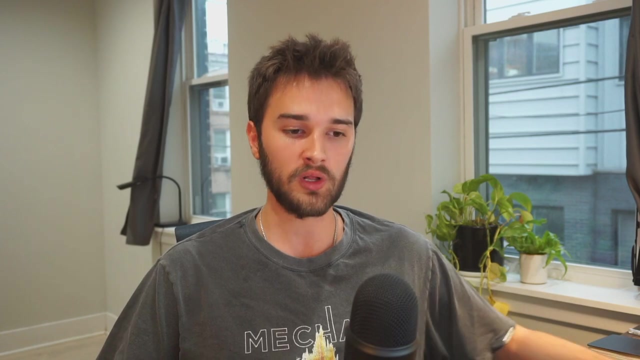 way back in the dizzy. okay, a long time ago this was for H-Com and something that nearly tripled the ROI of the ads overnight was not by coming up with some crazy new ad creative or some like untapped, like targeting opportunity or something or loophole. No, it was simply by 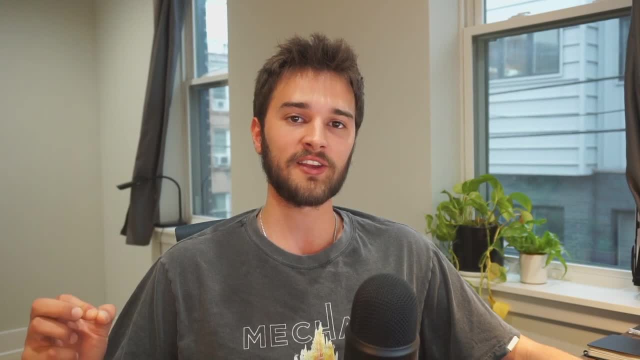 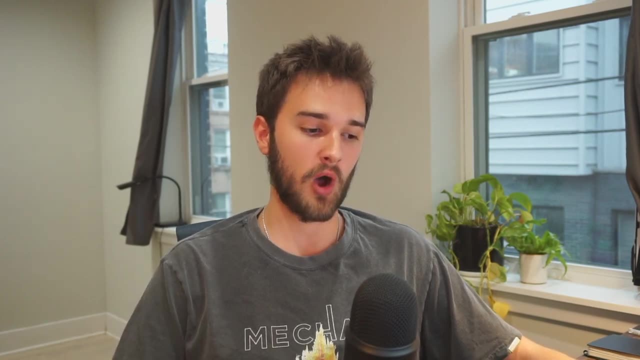 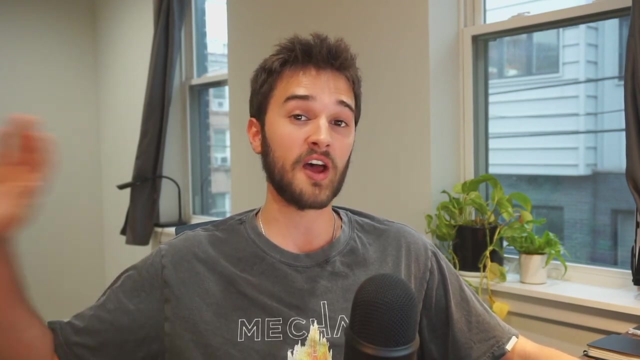 increasing the email deliverability rate so that more people would open the email and actually attend the damn webinar. That's a perfect example Of you could be fighting uphill day and night to try to increase your ad ROI. yet something that you know has nothing to do with ads, but also has everything to do with ads, is something that 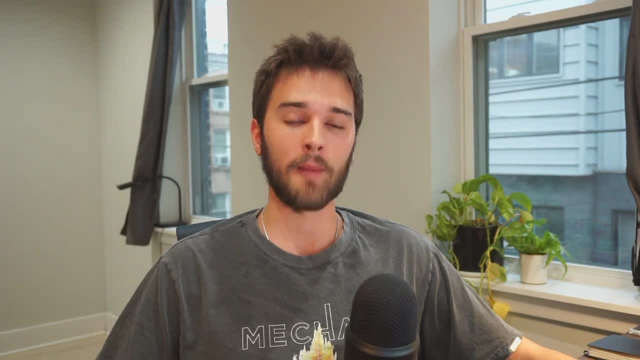 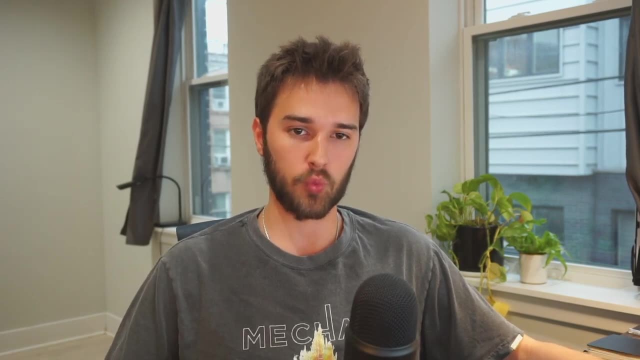 can increase the ad ROI by three times. You know, a button pusher media buyer is not going to see that, They're not going to understand that. And this is really what in my eyes, what a media buyer is and what it does. And again, this is coming from our media buyers as well. at 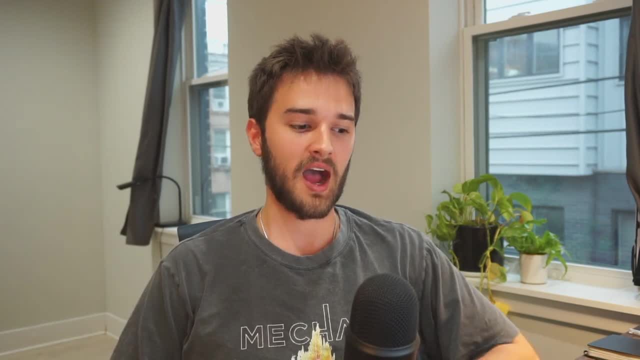 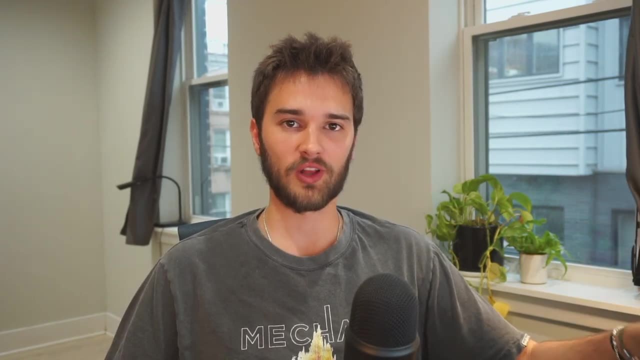 mediabuyercom in terms of what we see, What we doing, what we're doing And this is, in other words, kind of the shift that we're seeing in the market as well. So this is how we view our role and what we do, And not to digress or 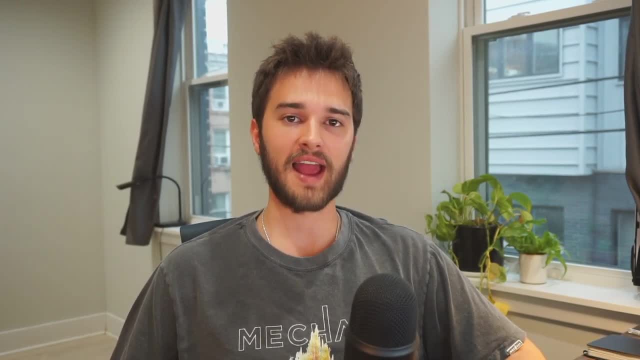 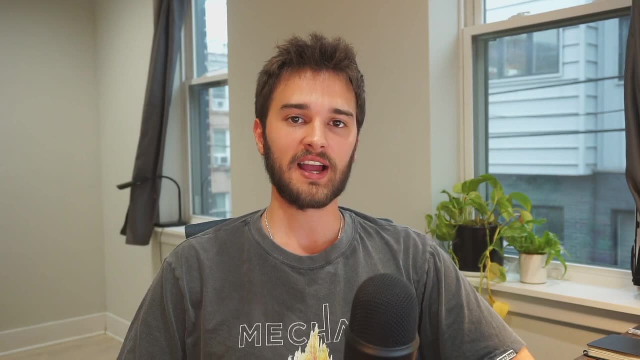 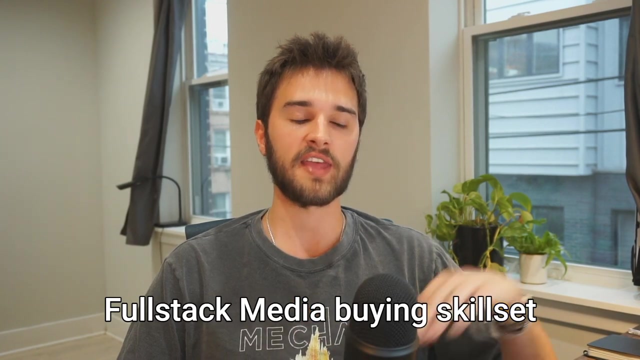 anything- because I'll make other videos about this in the future- but everybody and their grandma is telling you to start an agency or do SaaS, AI, all of these things. I think that the biggest untapped skill and opportunity is becoming a phenomenal media buyer. They are so rare out. 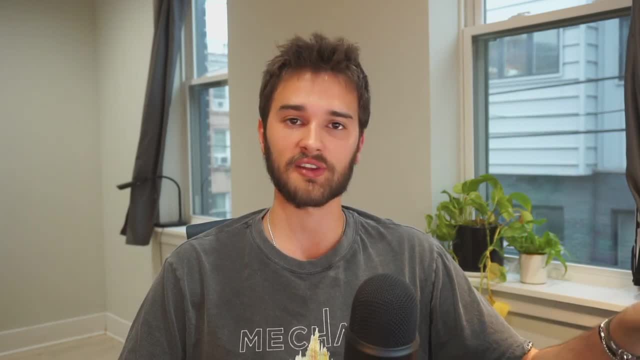 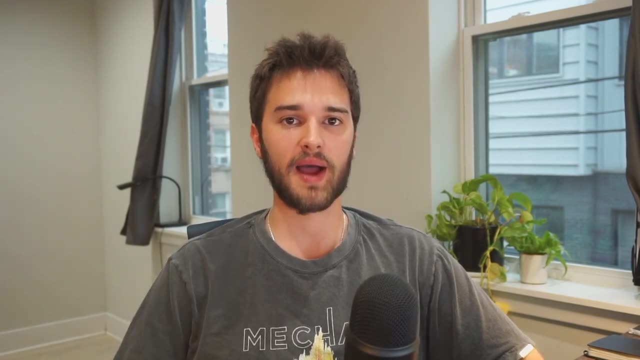